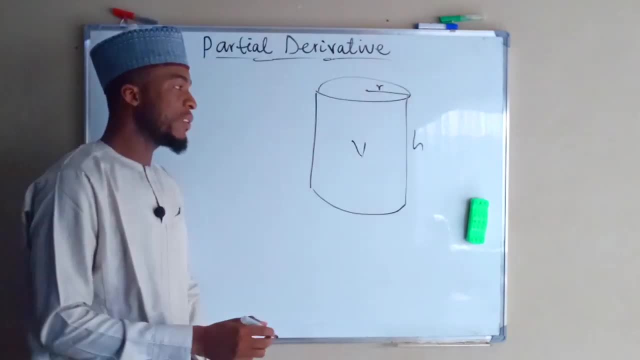 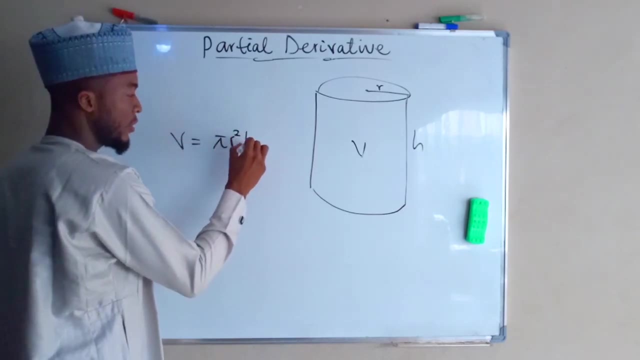 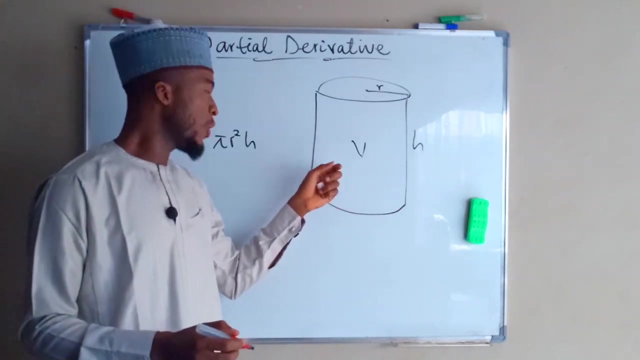 Suppose this is a cylinder. If this is a cylinder, the volume of this cylinder will be phi r squared h. Therefore, the volume depends on two quantities: the radius and height of this cylinder, While phi is constant here. So if the height of the 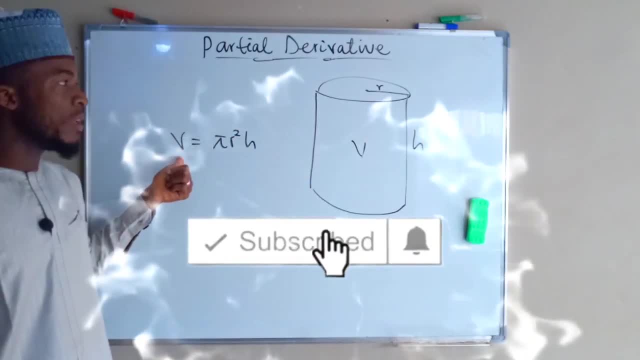 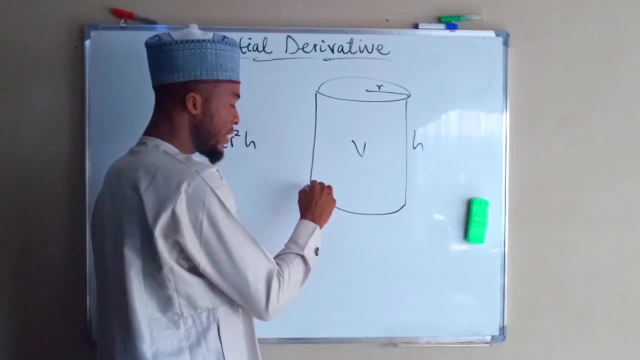 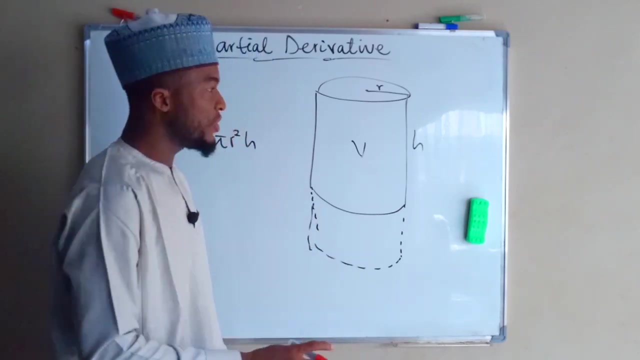 cylinder increases, also the volume is going to increase. At the same time, if the radius increases, also the volume is going to increase. If you increase the height of this cylinder, there will be a negative be change in height. there will be change in this h, which is height, as long as the height of this 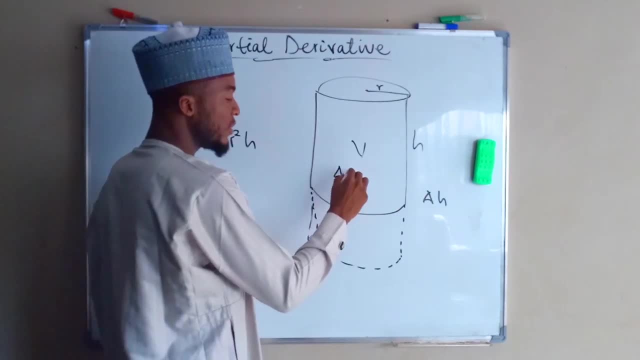 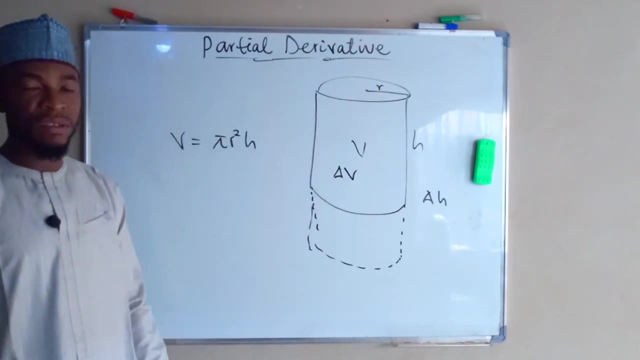 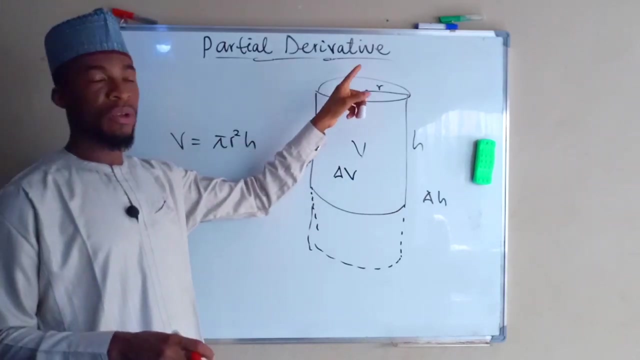 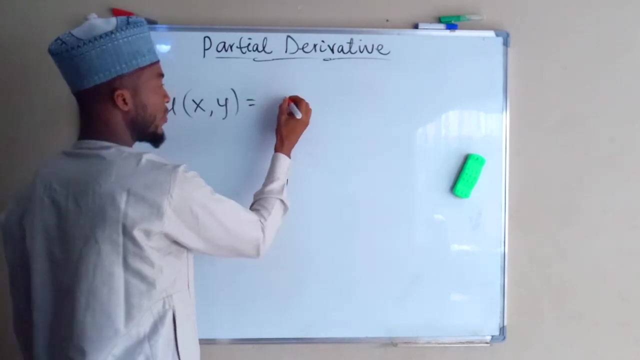 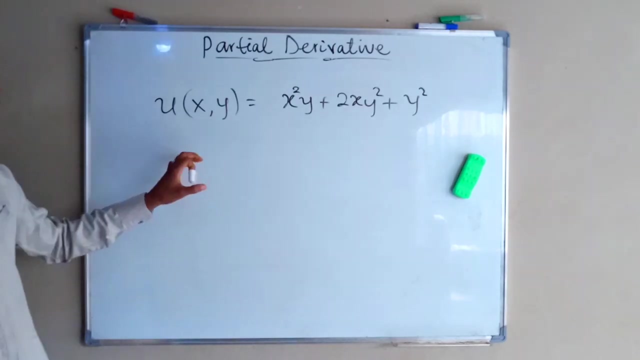 cylinder increase. also the volume is going to increase, while the radius remains constant. without increasing the volume of this radius, the volume of the cylinder increase. so therefore we can find the change in the volume with respect to height or with respect to radius. suppose u is a function of x and y, which is equal to this is a function u which defends on x and y. so you: 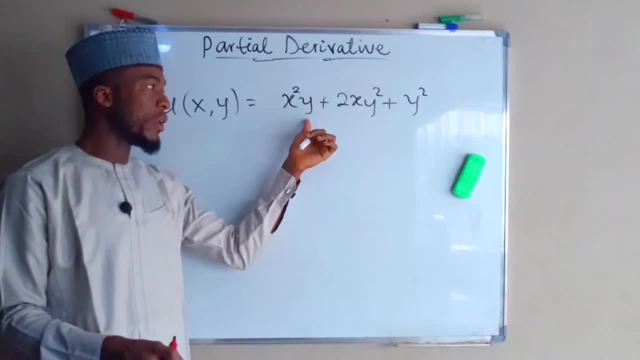 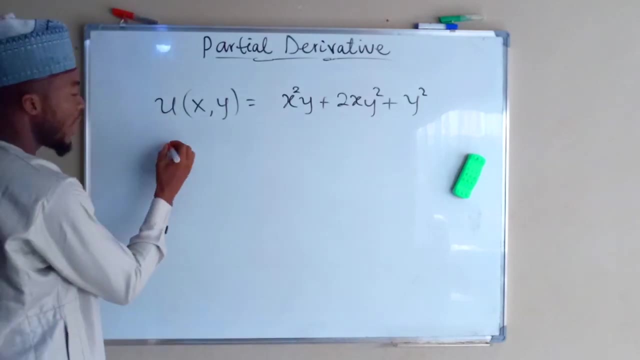 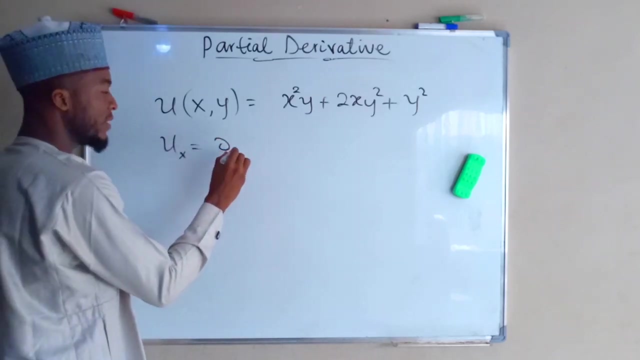 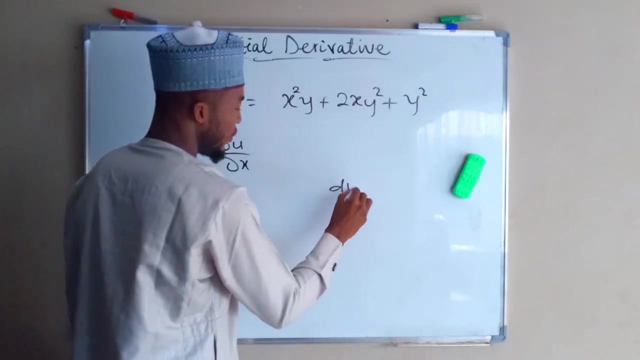 can differentiate this function with respect to either y or x. to differentiate u with respect to x, you are going to treat y as constant. therefore, we have use of script x, which is the same thing as, which is the same thing as delta u over delta x. this time around, we are not going to use the u over the x, because this: 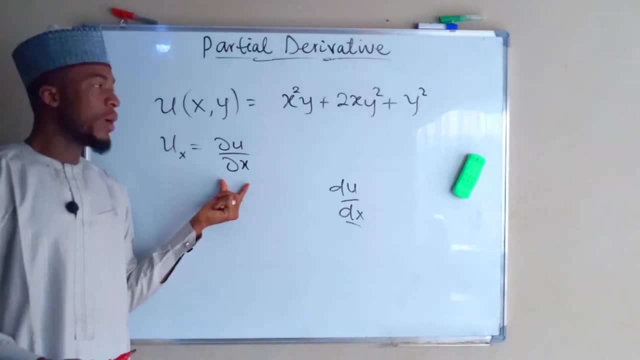 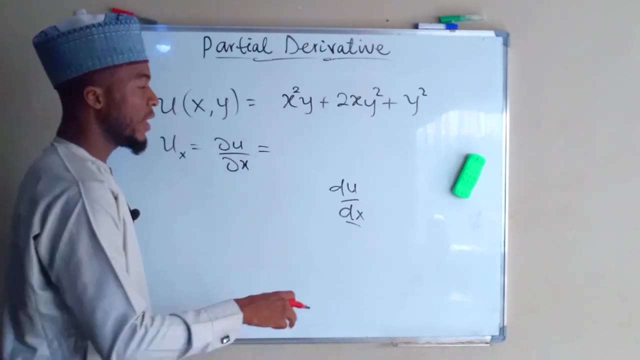 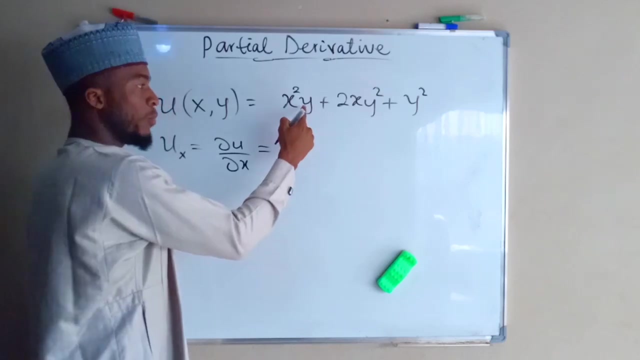 is total derivative, while this one stands for partial derivative. so we are going to differentiate this function with respect to x, treating y as constant. so if you differentiate x here you are going to obtain 2x. but remember y is constant, so we have 2xy. then the second term, if you. 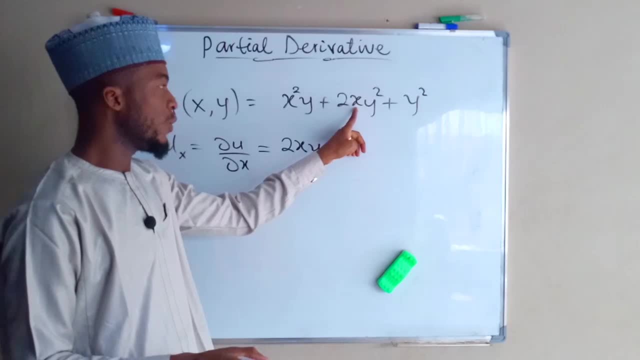 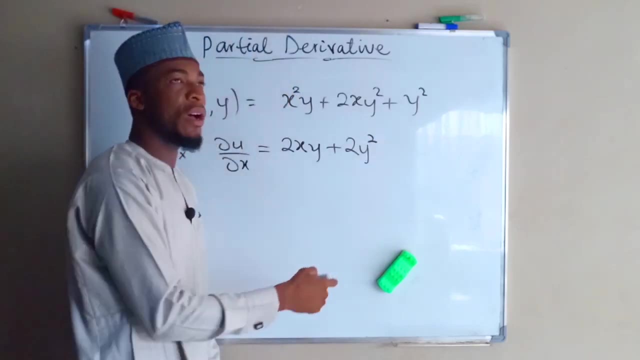 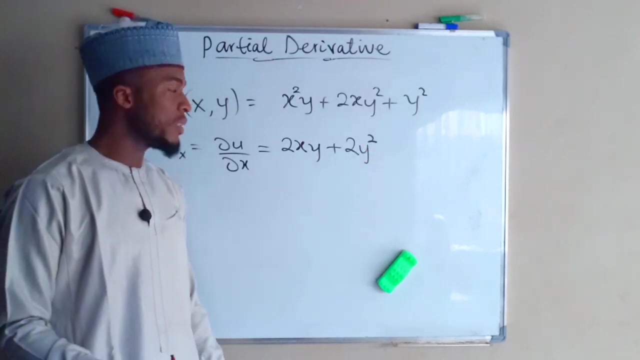 differentiate x. x has an index of one, so if you differentiate it it will vanish, leaving only 2y squared. and this- uh, the last term, does not contain any x, so you treat it as constant, but under you know that the derivative of a constant is zero. so this is the derivative of. 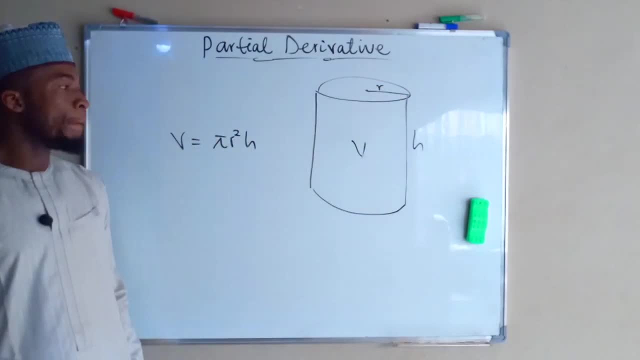 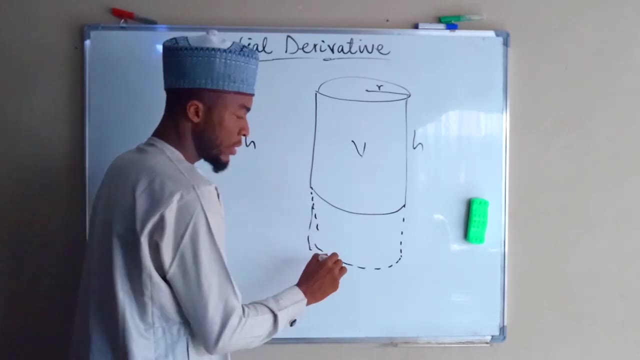 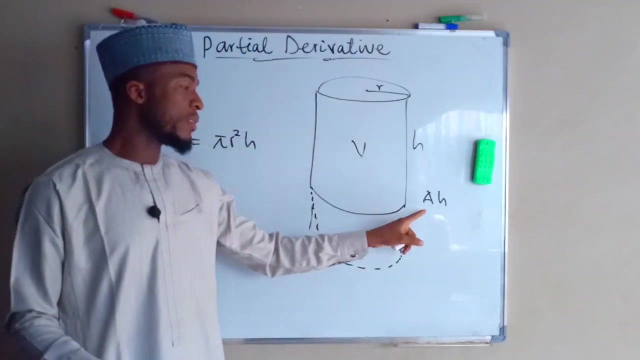 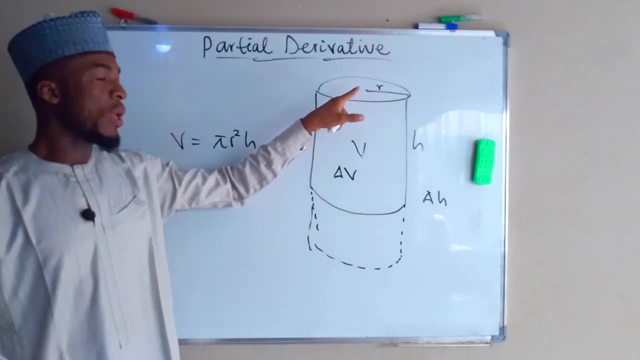 increases, also the volume is going to increase. If you increase the height of this cylinder, there will be more volume, be change in height. there will be change in this h, which is height. as long as the height of this cylinder increase, also the volume is going to increase, while the radius remains constant. 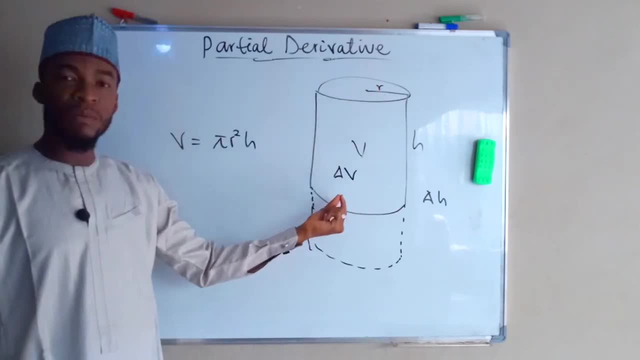 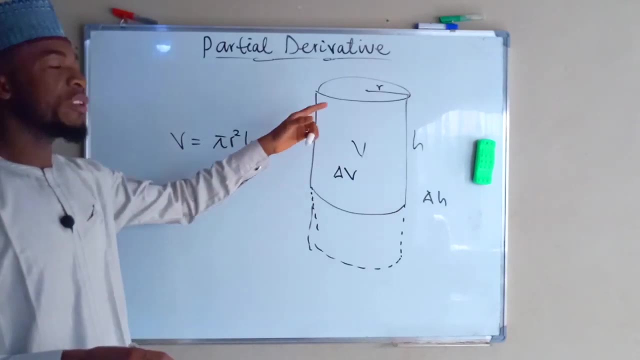 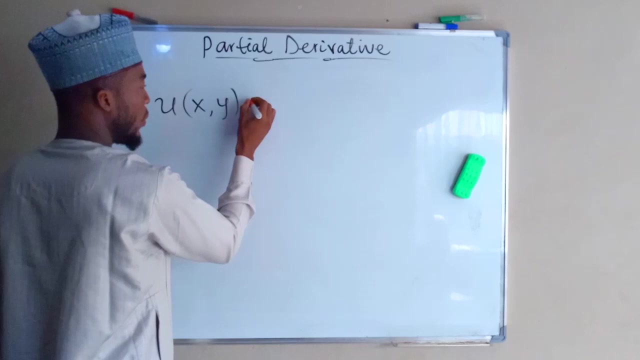 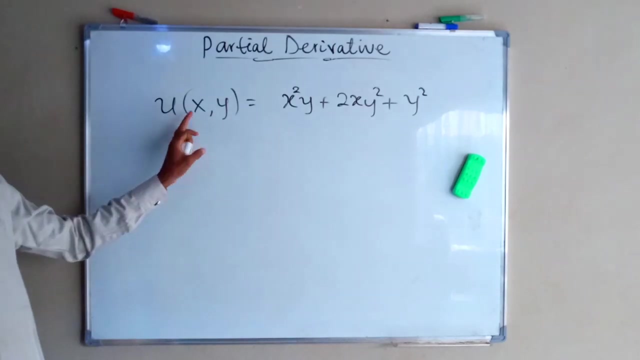 without increasing the volume of this radius, the volume of the cylinder increase, so therefore we can find the change in the volume with respect to height or with respect to radius. suppose u is a function of x and y, which is equals to it. this is a function, u, which depends on x and y. 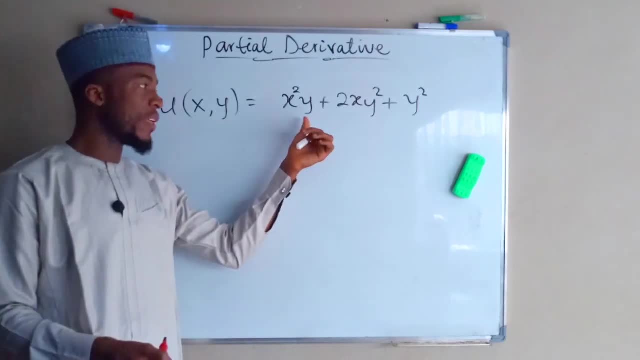 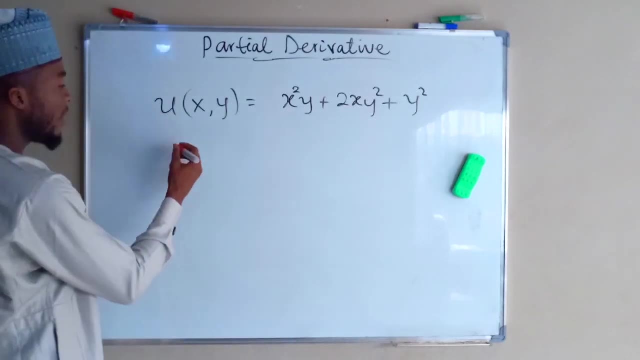 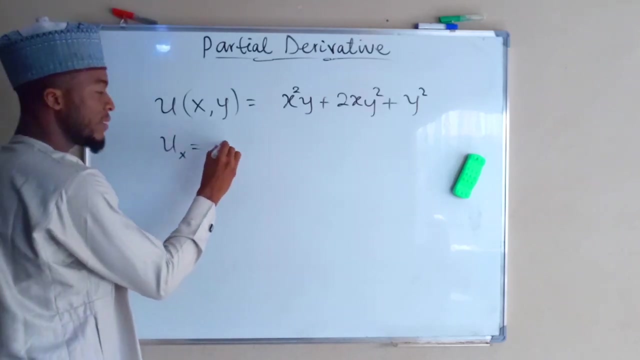 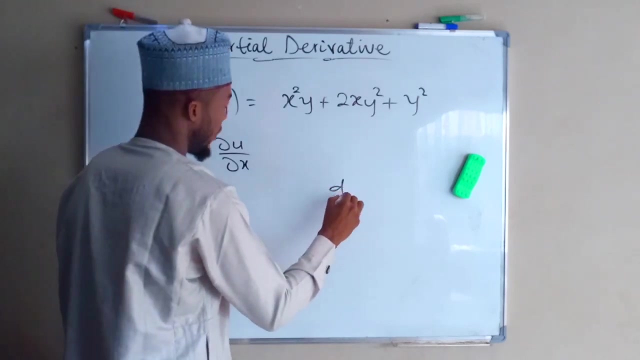 so you can differentiate this function with respect to either y or x. to differentiate you with respect to x, you are going to treat y as constant. therefore, we have use of script x, which is the same thing as, which is the same thing as delta u over delta x. this time around, we are not going to use the u over the x, because this: 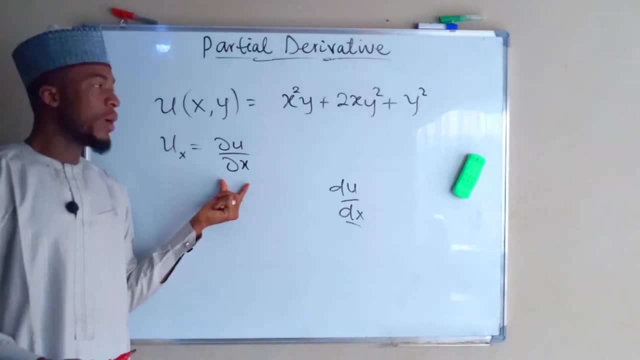 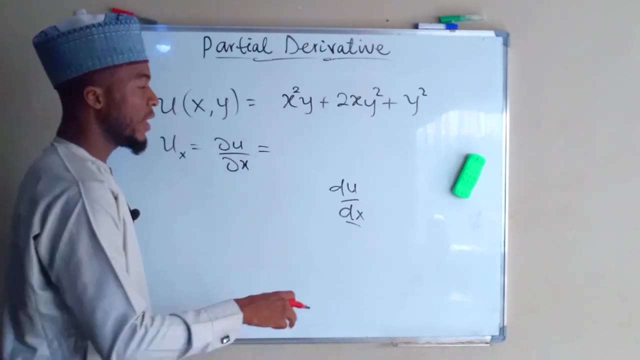 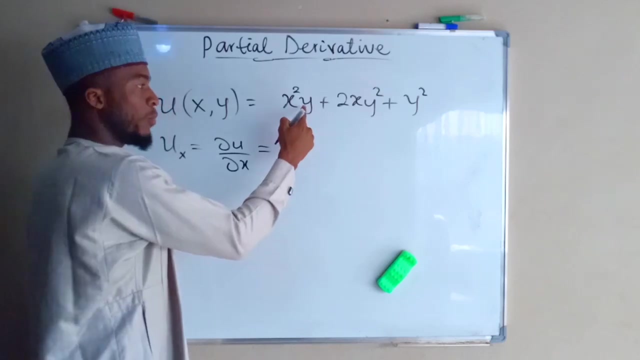 is total derivative, while this one stands for partial derivative. so we are going to differentiate this function with respect to x, treating y as constant. so if you differentiate x here you are going to obtain 2x. but remember y is constant, so we have 2xy. then the second term, if you. 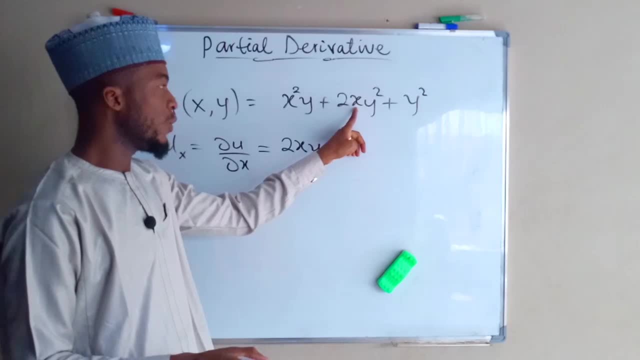 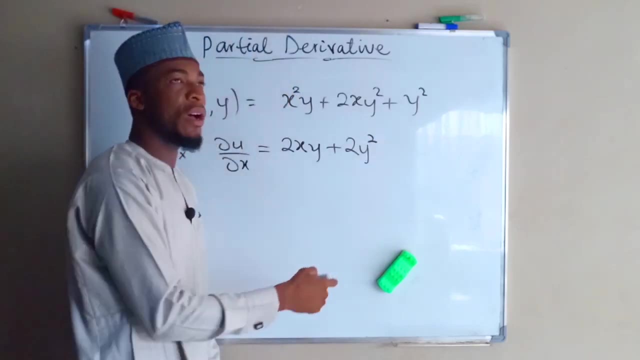 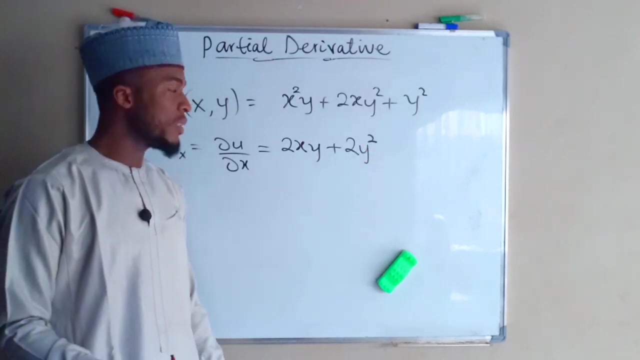 differentiate x. x has an index of one, so if you differentiate it it will vanish, leaving only 2y squared. and this- uh, the last term, does not contain any x, so you treat it as constant, but under you know that the derivative of a constant is zero. so this is the derivative of. 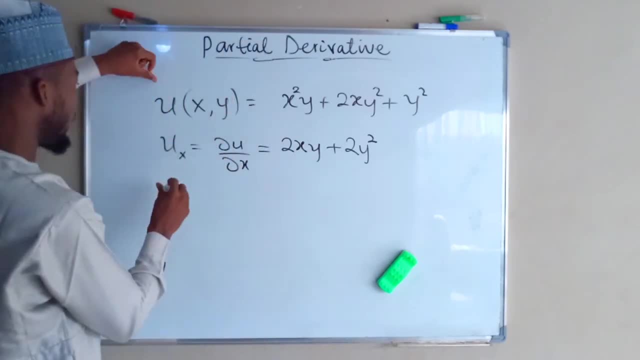 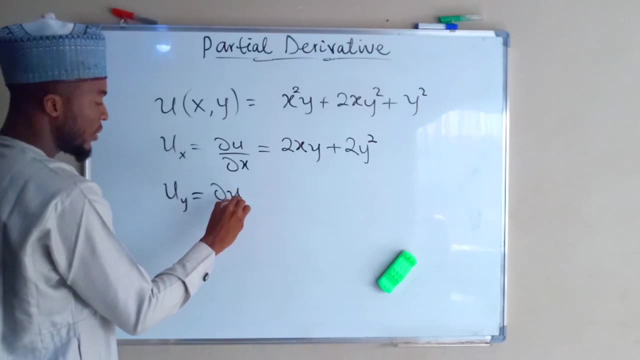 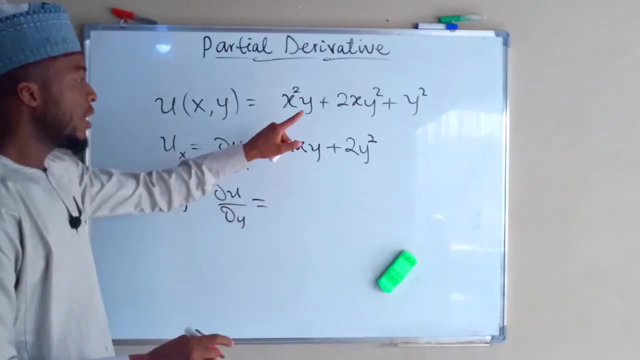 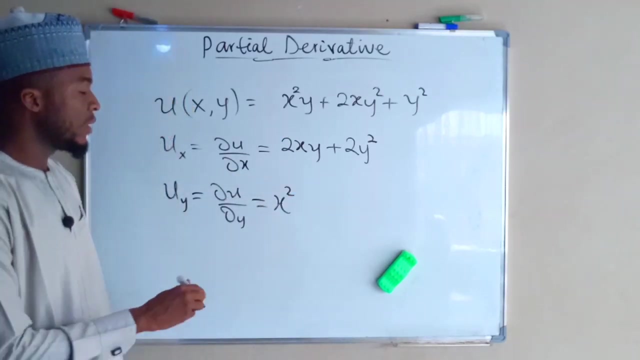 you u with respect to x. now to differentiate u with respect to y, you are going to differentiate du over dy, keeping x as constant, and this will result to: if you differentiate y here, you are going to get one one times: x squared is the same thing as x squared plus the second term. 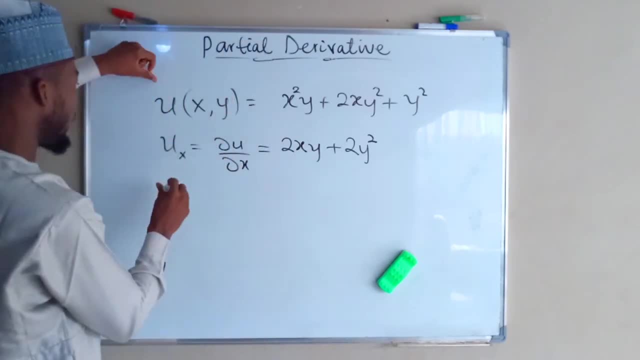 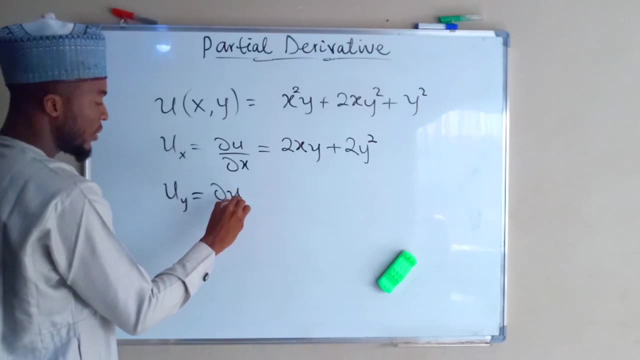 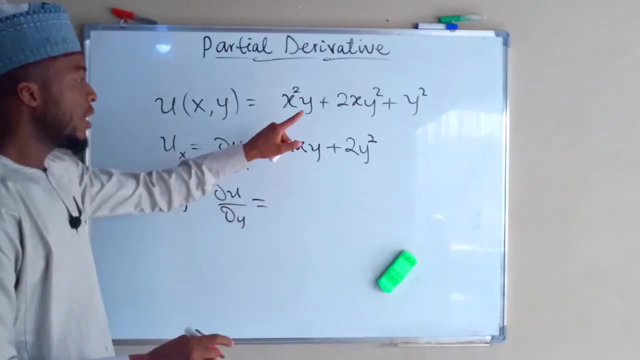 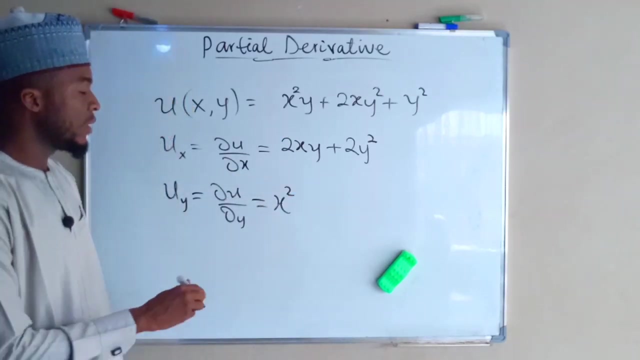 you u with respect to x. now to differentiate u with respect to y, you are going to differentiate du over dy, keeping x as constant, and this will result to: if you differentiate y here, you are going to get one one times: x squared is the same thing as x squared plus the second term. 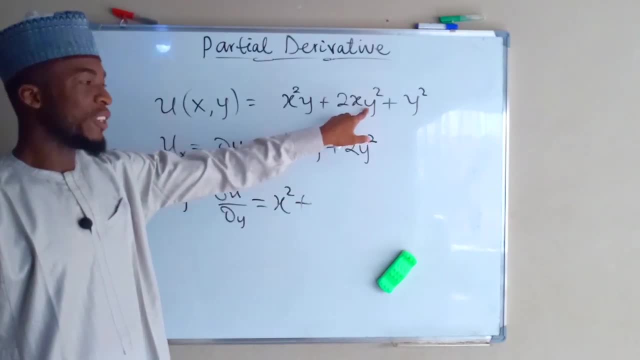 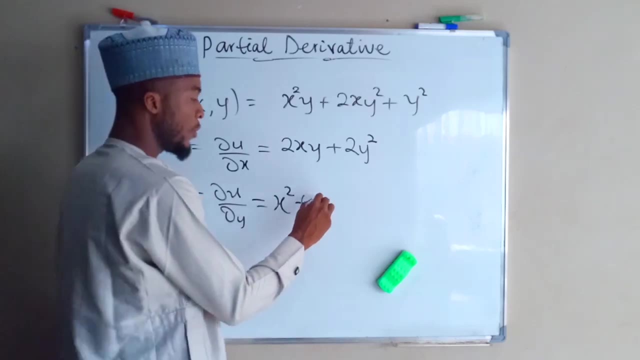 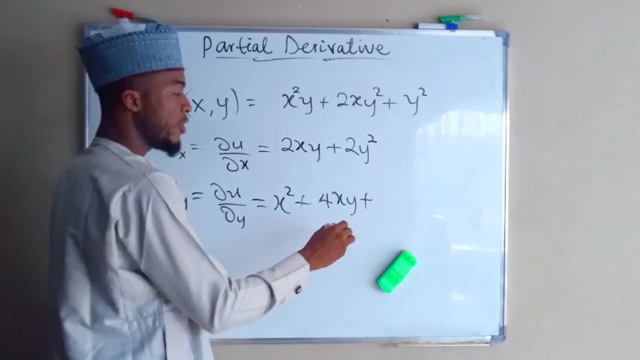 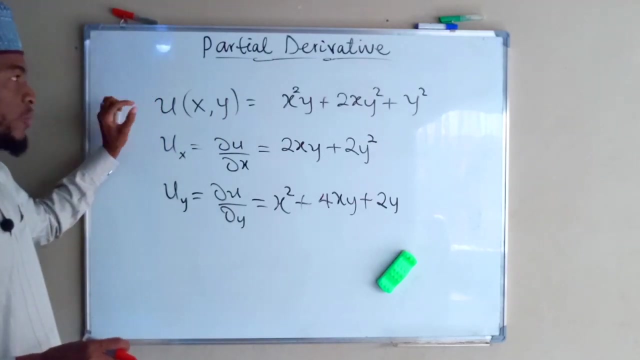 if you differentiate this, you are going to obtain 2y. remember the other coefficient remains constant. so we have 2y times 2x, making 4xy. plus if you differentiate the last term, which is also y, we are going to obtain 2y. so this is how to differentiate a function. using partial derivative, you can differentiate. 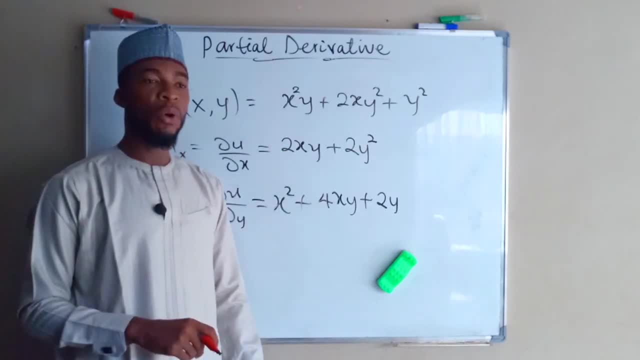 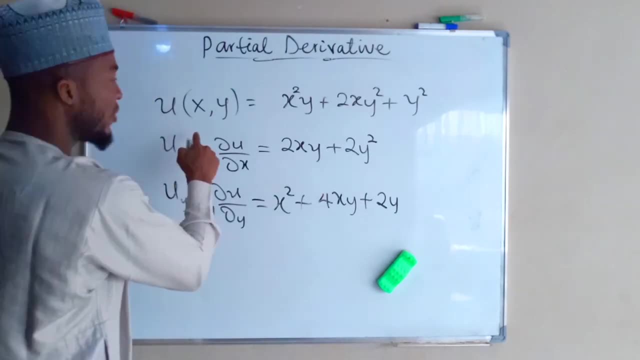 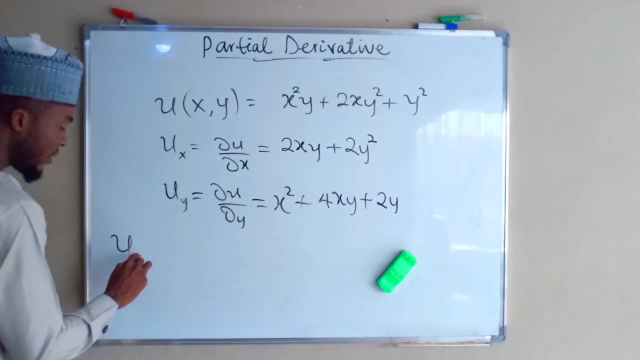 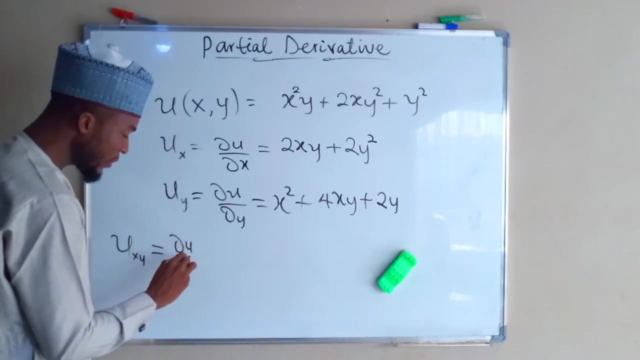 that function with respect to one of the variables, or you can differentiate it with respect to all the variables. so now, if we are to differentiate this with respect to x and y together, what i mean here is you soft script x, y. this is the same thing as uh saying du over dx. 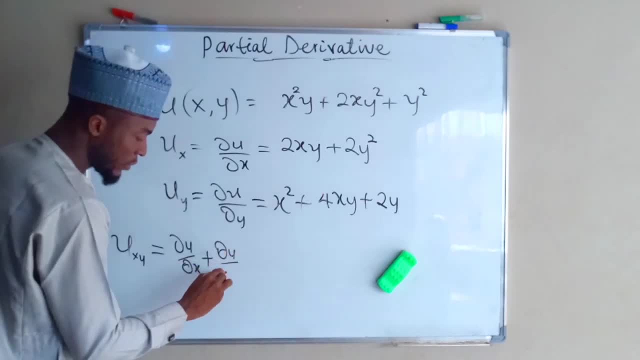 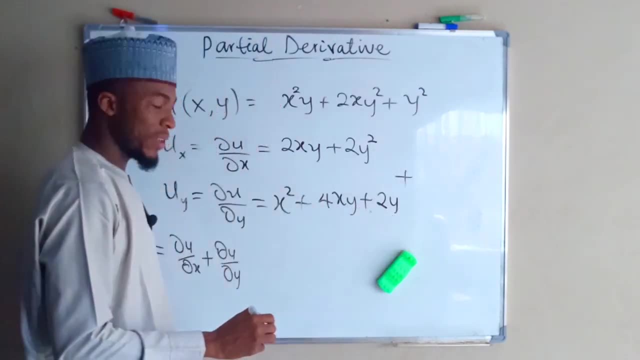 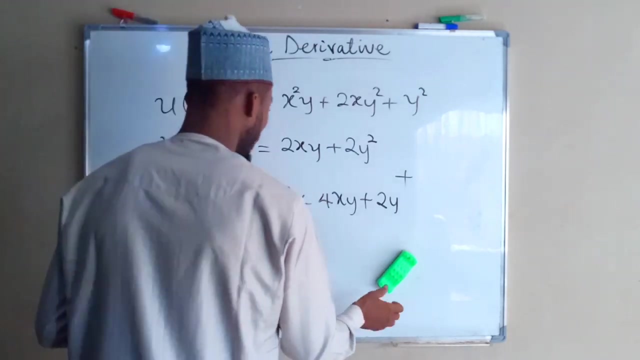 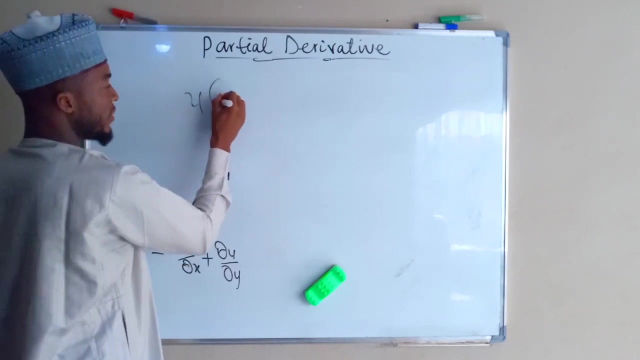 plus du over dy. so in this case you are only going to add these two times together in order to obtain this derivative. at the same time, if you are given a trigonometric function, you can apply the same principle. suppose you have u which depends on x and y equals. 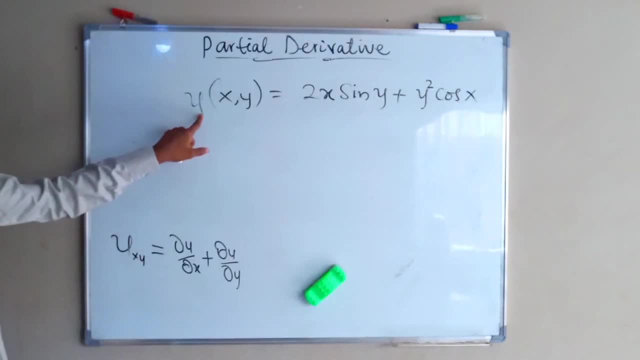 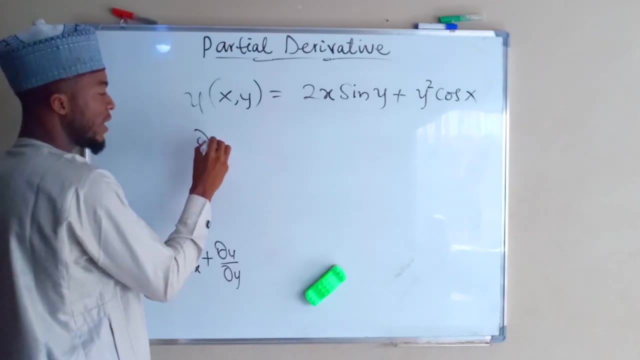 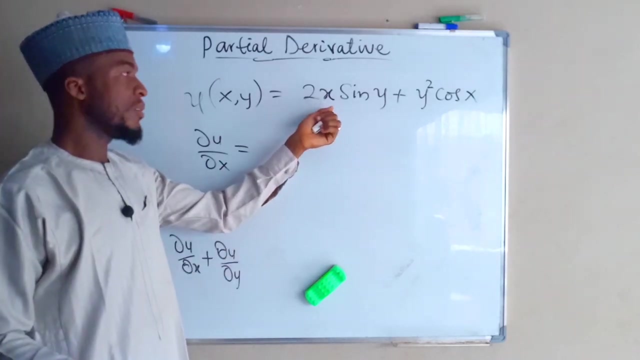 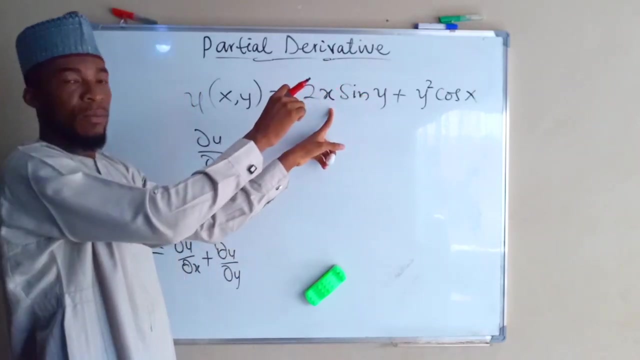 if you want to differentiate this function with respect to X, you are going to differentiate x treating y as constant. so we have Delta u, Delta x equals in the first time. we have X. so we are differentiating with respect to X. so you are going to differentiate X treating all other quantities as constant. 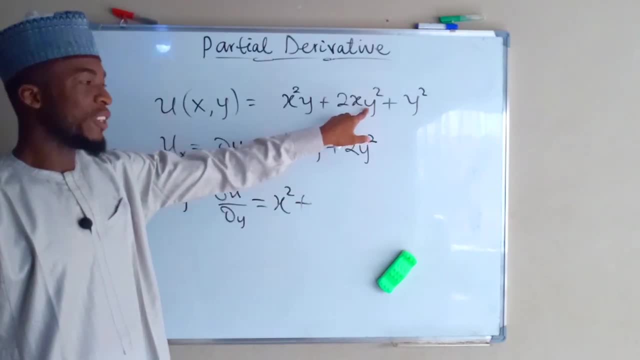 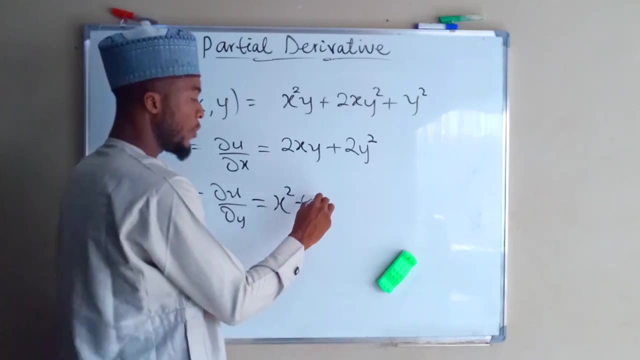 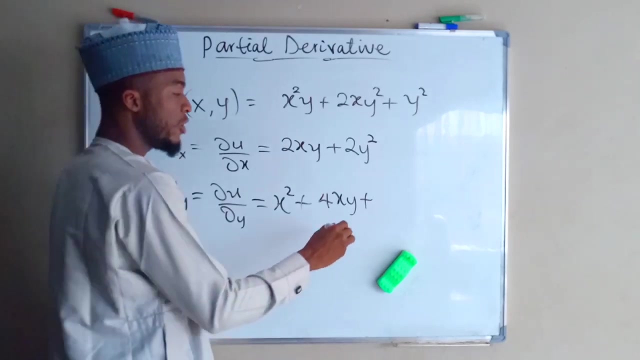 if you differentiate this, you are going to obtain 2y. remember the other coefficient remain constant. so we have 2y times 2x, making works 4x. y. plus, if you differentiate last time, which is also y, we are going to obtain 2y. so this is: 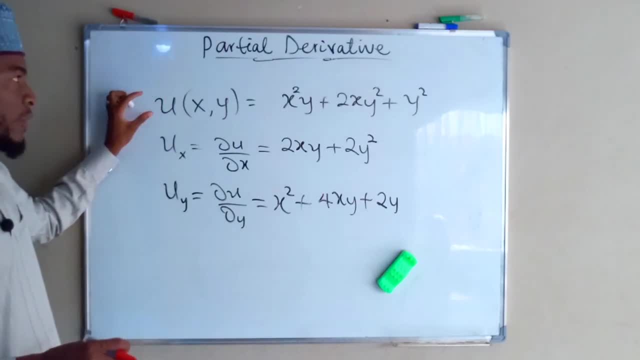 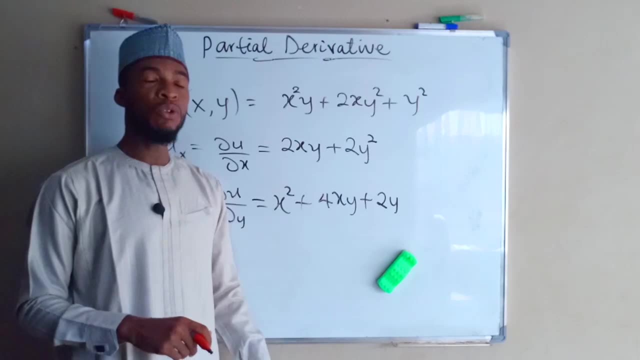 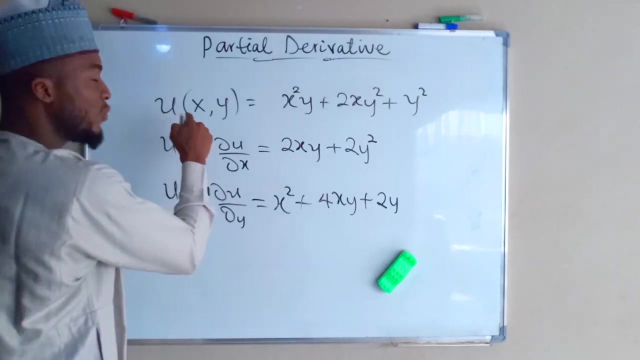 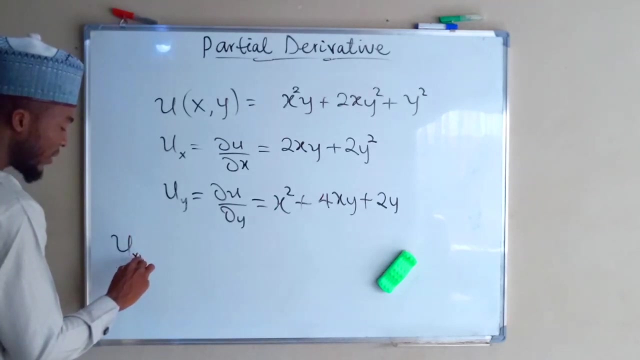 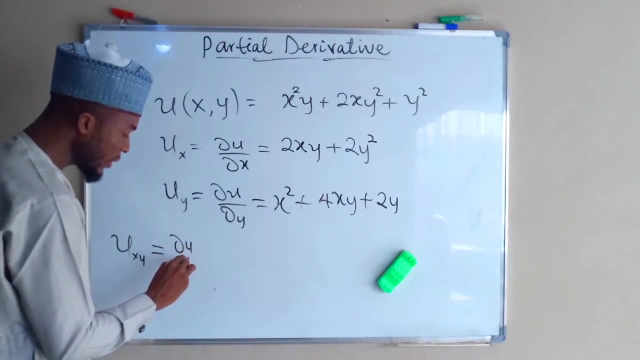 how to differentiate a function using a partial derivative. you can differentiate that function with respect to one of the variables, or you can differentiate it with respect to all the variables. so now, if we are to differentiate this with respect to x and y together, what i mean here is u subscript x, y. this is the same thing as saying du over dx. 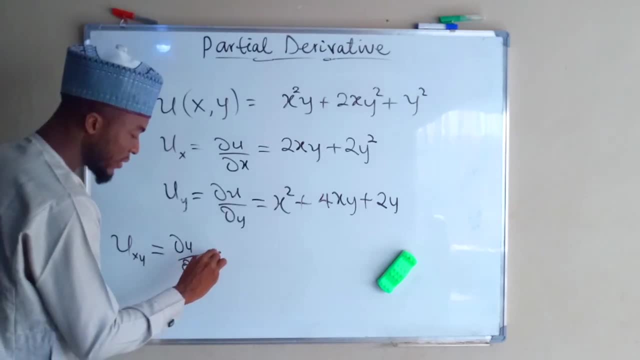 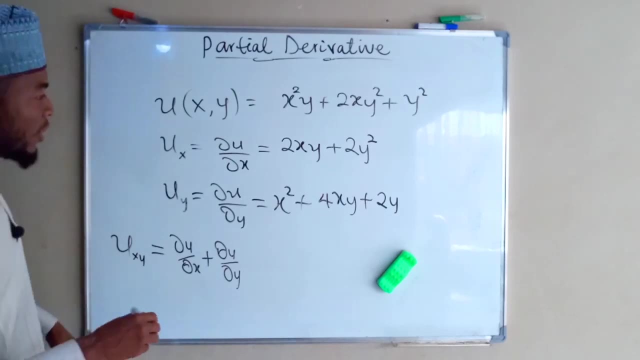 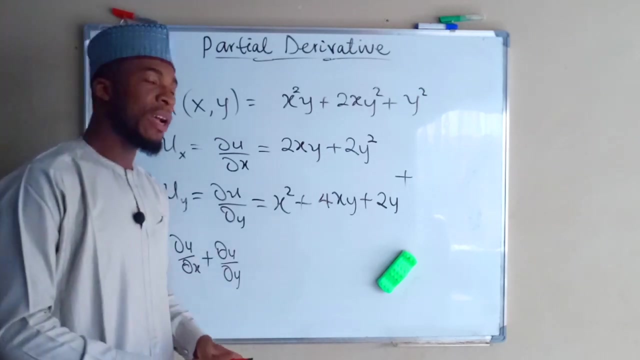 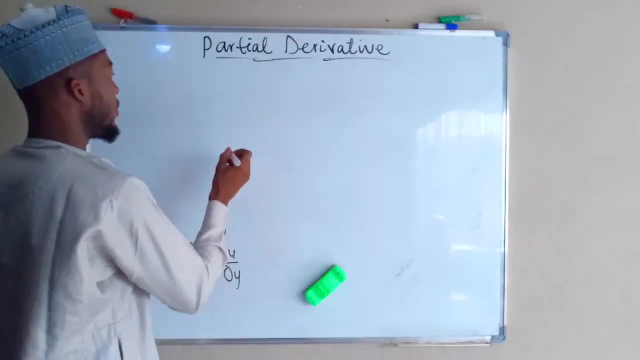 plus du over dy. so in this case you are only going to add these two times together in order to obtain this derivative. at the same time, if you are given a trigonometric function, you can apply the same principle. so suppose you have u which depends on x and y. 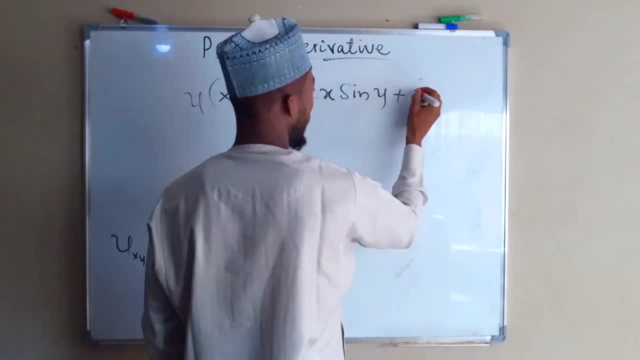 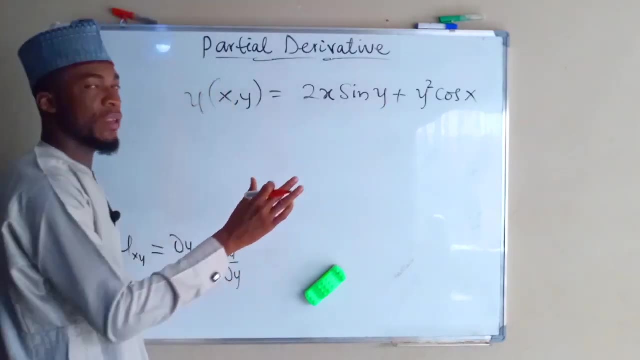 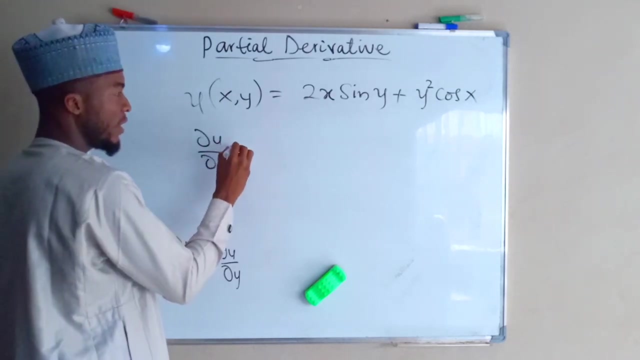 is Because, if you want to differentiate this function with respect to x, you are going to differentiate x, treating y as constant. So we have delta u, delta x equals and the first time we have x. so we are differentiating with respect to x. 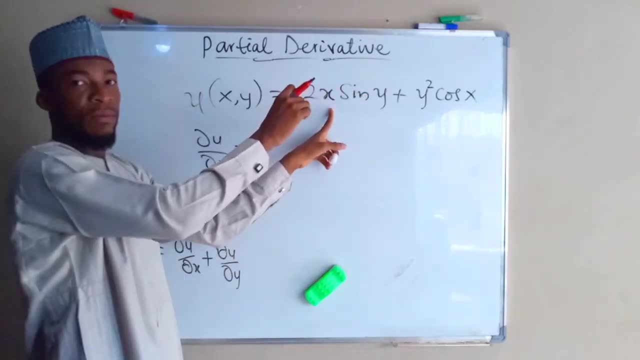 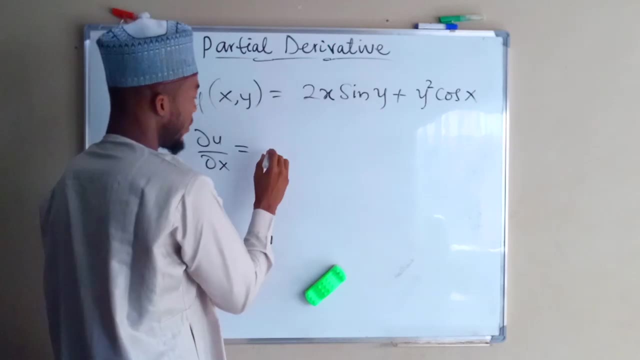 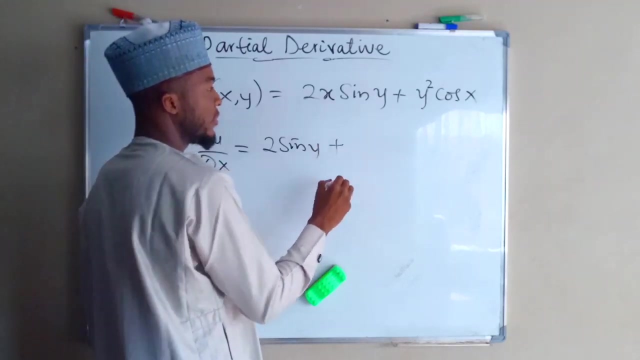 So you are going to differentiate x, treating all other quantities as constant. So if you differentiate x, you are going to obtain 1, leaving only 2 sine y. So we have 2 sine y, Plus you keep this constant. you differentiate this. 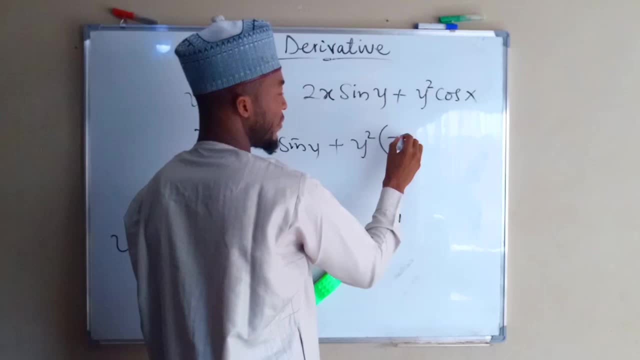 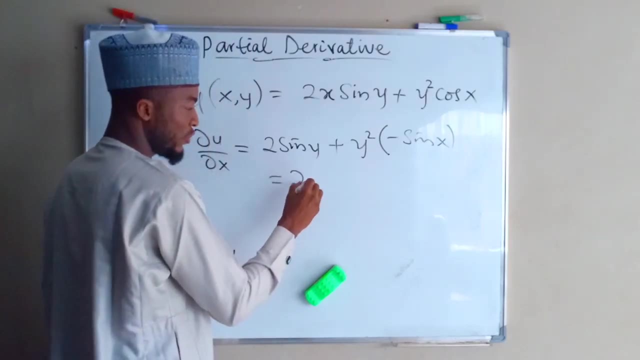 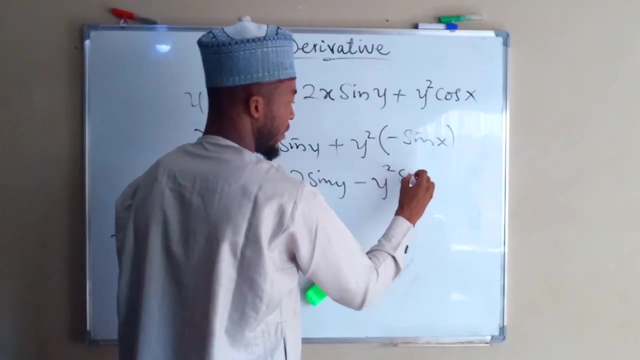 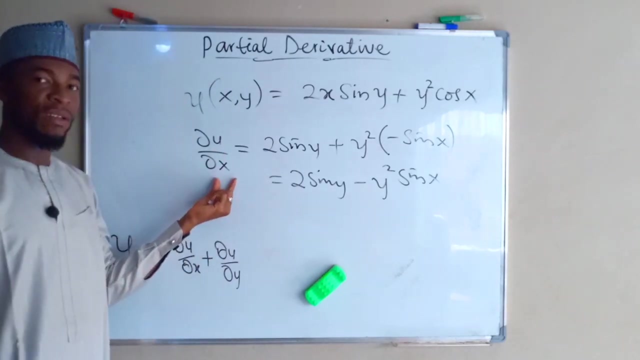 This remains constant. If you differentiate this, you are going to obtain minus sine x, And this altogether equals to 2 sine y Minus y squared sine x. So this is the derivative of this function with respect to x, keeping y as constant.